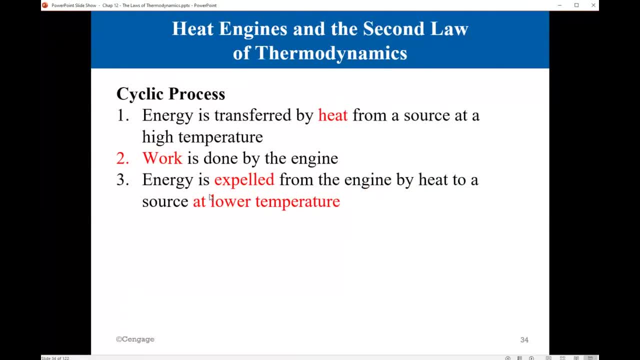 We move on to heat engines and the second law of thermodynamics. We have cyclic process and also we have Carnot engines to discuss when we talk about the second law of thermodynamics. In a typical cyclic process, energy is transferred from the environment to the system, so the system takes heat and the 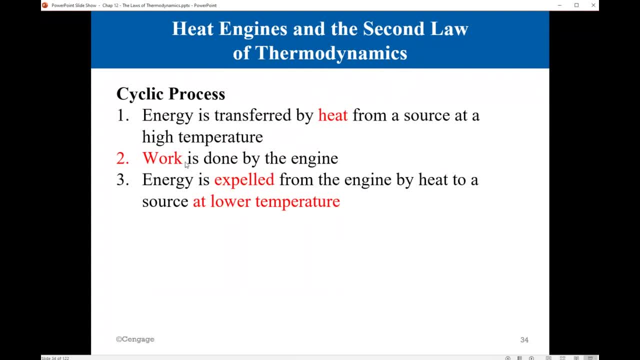 system performs work. Part of this heat is used to do work and the other part is expelled to the surrounding, which is at a lower temperature from the original heat source, For example in our cars by burning gasoline in the engine. that is the source of the heat, Part of that. 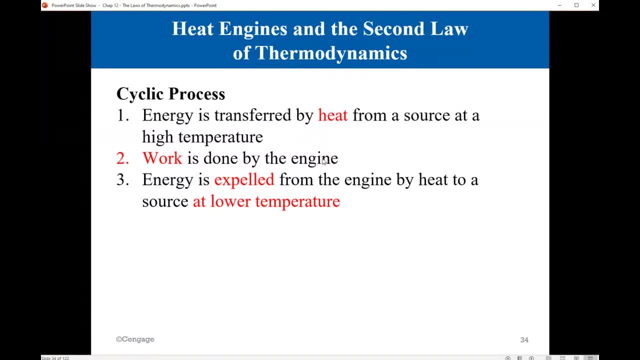 heat is used to do mechanical energy to move the car, and the remaining part is expelled through the exhaust to the surrounding, which is the atmosphere, which is at lower temperature than the temperature of the engine. That is a typical system. That is a cycle that repeats over and over again. So we have 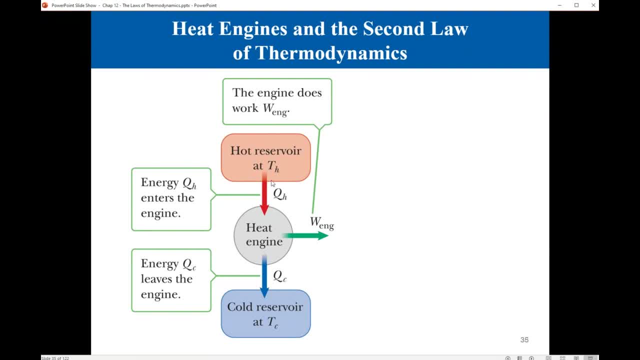 hot reservoir at temperature TH, where the system takes quantity of heat, QH, The engine performs work for the car engine, it does mechanical motion and there is an amount of energy being expelled to the surrounding. we call it the cold reservoir. So we deal with a hot reservoir and a cold reservoir. the temperature for the 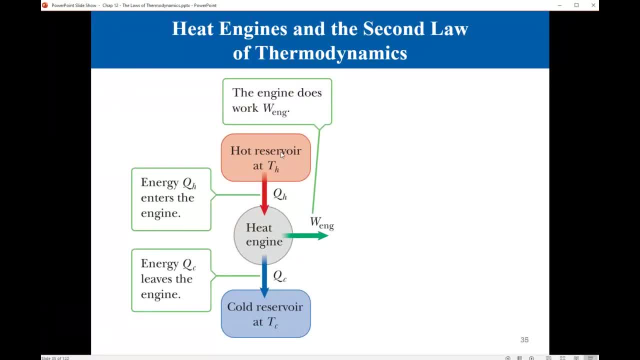 cold reservoir it is less than the temperature for the hot reservoir. always, The change in the internal energy for this cyclic process is zero. therefore, Q equals minus W and the Q here is the net difference between QH and QC. We are interested in the net heat energy. This is the one that is related to the 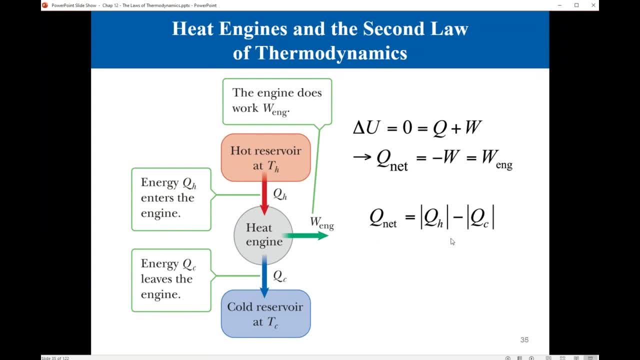 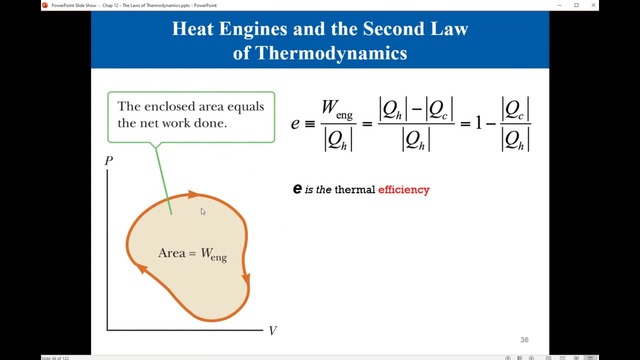 work done by the engine. So the difference between QH and QC, Q net is equal to the work done by the engine. Here this area represents the cycle, So the area in the PV diagram is equal to the work done by the engine. 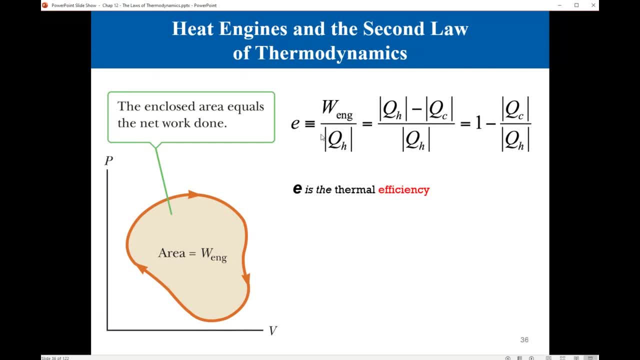 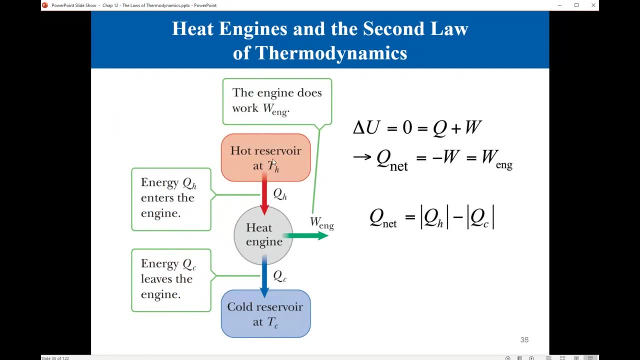 The efficiency of the heat engine is equal to the work the engine divided by a QH If you go back. so this is the output, this is the output, this is the input, this is the waste. So the efficiency there. 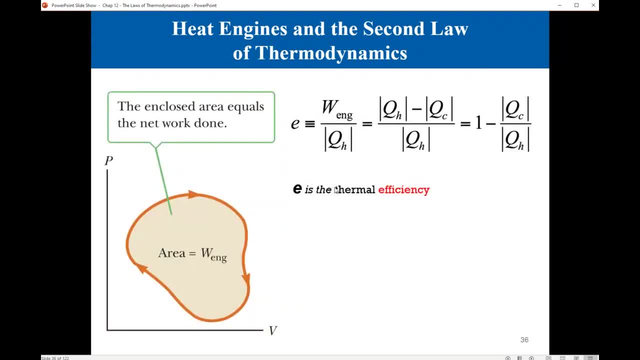 the output. This is the input, this is the waste energy divided by the input energy. This is how we define the efficiency And the work done by the engine is the difference between QH minus QC. So here you have QH minus QC. divided by QH Simplify, this is equal to 1 minus QC. 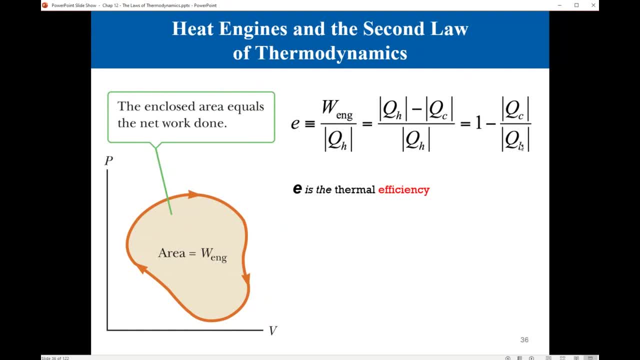 over QH. QC is always less than QH, so this is a fraction. 1 minus fraction is another fraction. so this tells us that the efficiency will always be a fraction. it will never be one. it will always be sure than one. This is called. 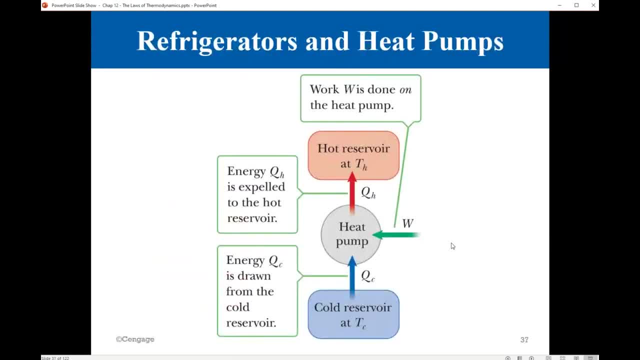 the thermal efficiency of the heat engine. The heat pump is also a heat engine, but it operates in a different way. Like All, there is a heat pump There. the heat pump takes the energy from the cold reservoir and dumps that energy to the hot reservoir Inside the refrigerator. it's cold, It takes. 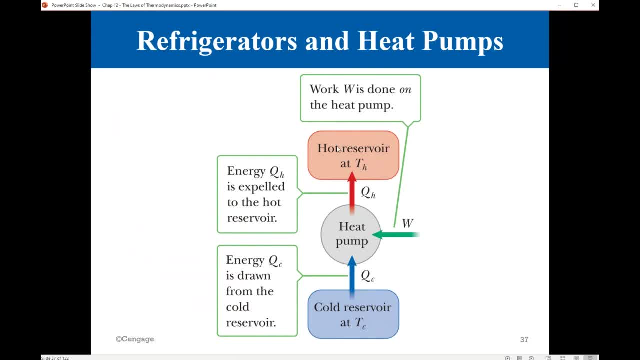 energy from the cold reservoir and dumps it to the surrounding, which is the hot reservoir. Of course, this will never happen spontaneously. This will never happen by itself. In order for this to happen, we need to provide mechanical energy, mechanical wear from an 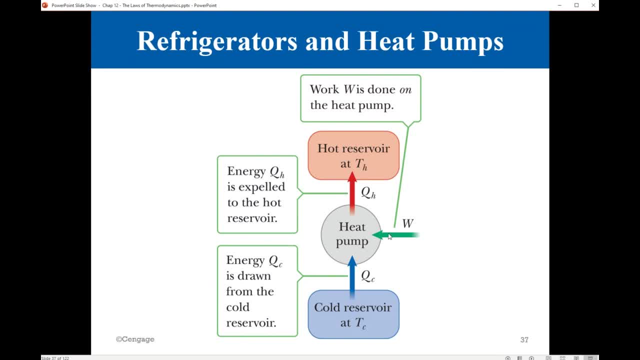 outsized source. So the motor of the refrigerator here uses electric energy to take the energy from the cold reservoir at temperature Tc and dump it to the hot reservoir at temperature Th. So as you can see here, this engine will never work by itself except if you provide the needed. 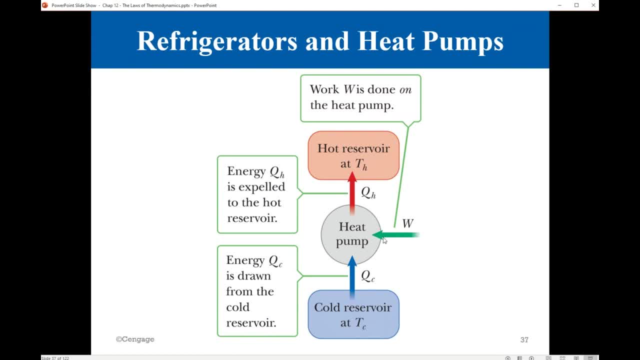 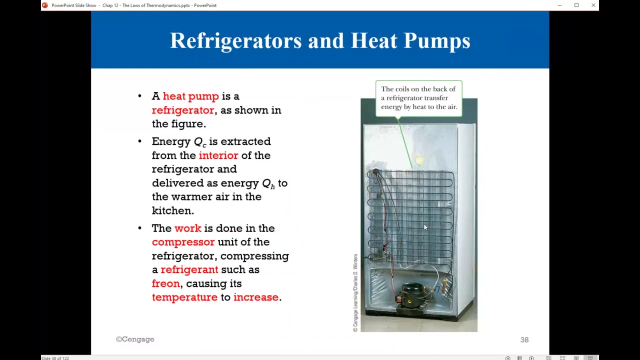 work from this internal source. The same model applies to air conditioning, also the ACs. They are also the same thing. We provide work from the electric outlet. If you connect two batteries to the natural gas Afterigten heat, we can easily protect the炎ro Water inside the water. 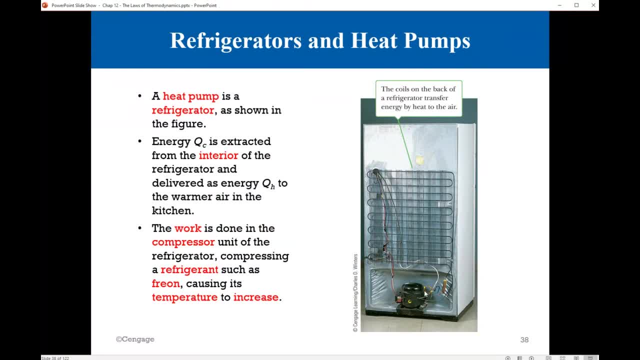 Thus we also receive electric energy from the cold reservoir. The critical part of class is temperature. We have these three problems. The first one is the problem of having a non-候ling heat pump turning on one direction so that the substances entering the reactor original system and energy such that theinton. diye sorrt we are able to take from the cold reservoir to down is available Second to so. this is an example of the Heath pump, the freige. we see so the heat pump, the refrigerator. we see how this motor takes electricity from the core outlet. 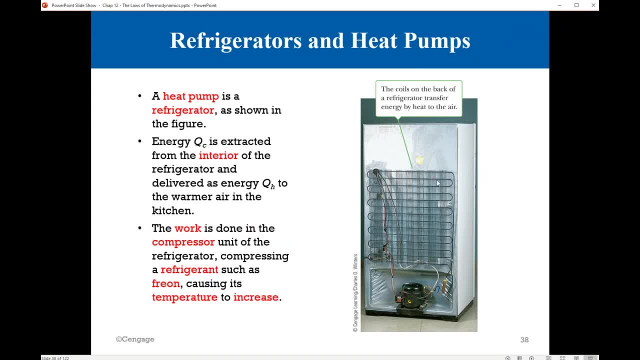 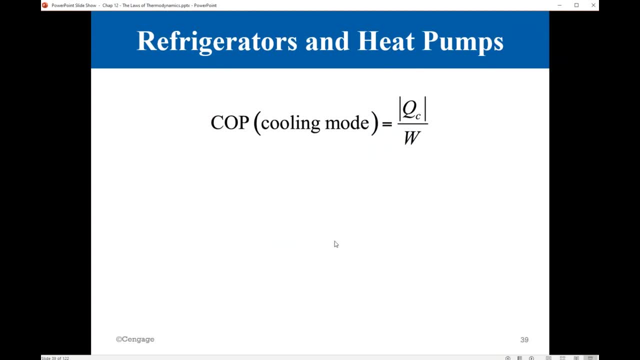 and exerts work over the gas such that it's able to move heat energy from the cold reservoir in a single stack. Stiff determine that large returns to the heat steam is continent reservoir inside and emit it to the surrounding which is at a higher temperature. 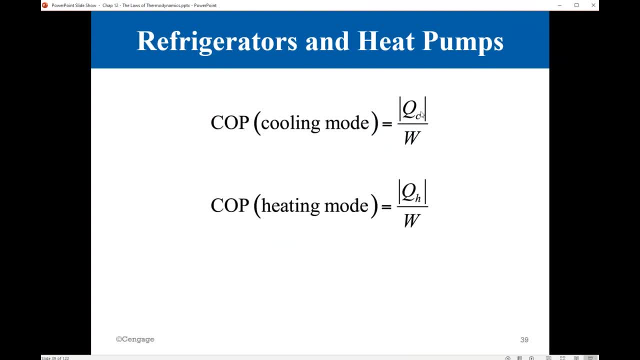 The efficiency for the cooling mode is QC divided by W. The efficiency for the heating mode for the heat pump, is QH divided by W. So, as we see, the efficiency is always less than one. The efficiency will never be equal to one. 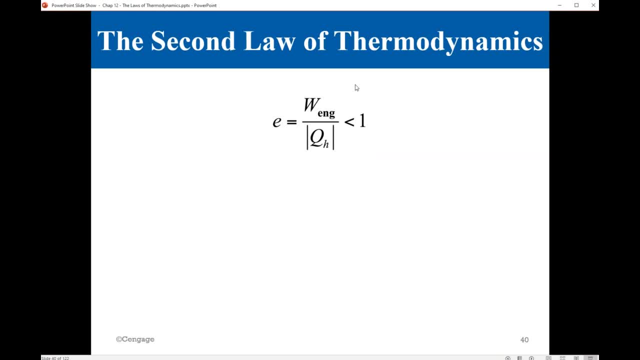 This is the difference between the second law and the first law of thermodynamics. The first law of thermodynamics speaks about energy conservation: That whatever energy is given to the system, it will appear in the form of work or change in the internal energy. 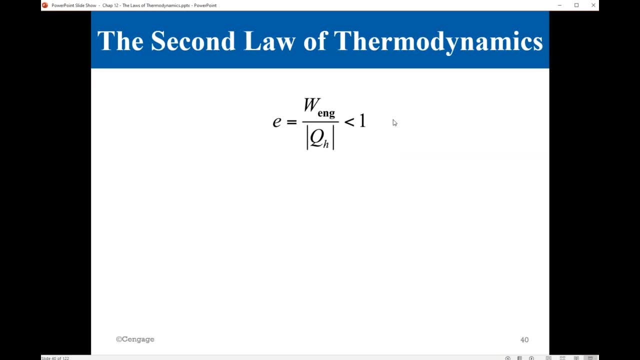 Energy is conserved. But here the second law of thermodynamics tells us that no matter what we do, the energy we do, we cannot get a work equal to the input energy, QH. There will always be waste energy released to the environment. 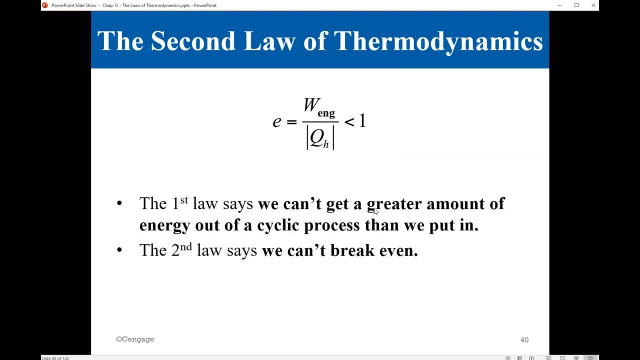 So this is a constraint on the first law of thermodynamics. So the first law says we cannot get a greater amount of energy out of a cyclic process than we put in. That's the energy conservation. But the second law says we cannot break even because always the energy output will be less. 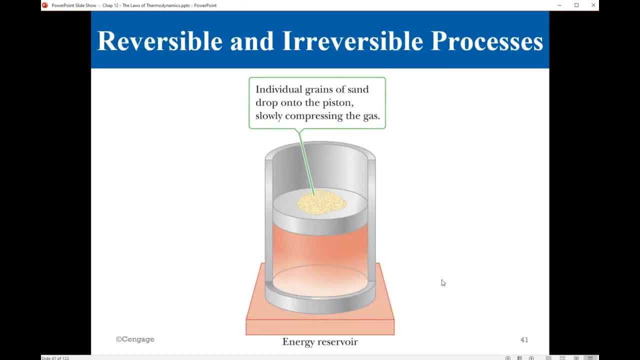 than the energy input. Another topic that we need to learn about is the reversible and the irreversible process. By a reversible process, we mean to take a system from one to another And bring it back to the original state. In reversible, this means that it is not possible to retain the system to its original state. 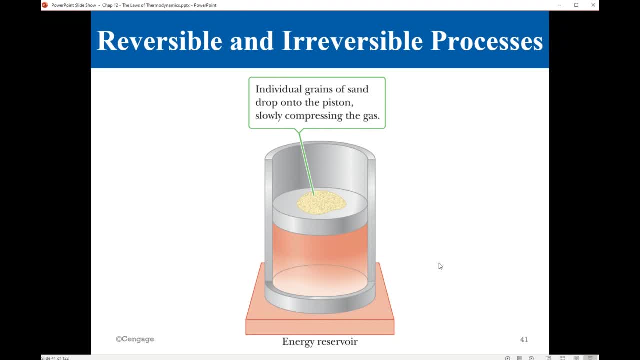 Consider, for example, the car engine that we are talking about. In the car engine, part of the heat energy is used to do mechanical work, to move the car, And the other part is to remove the exhaust That is due to the mechanical work of the car. 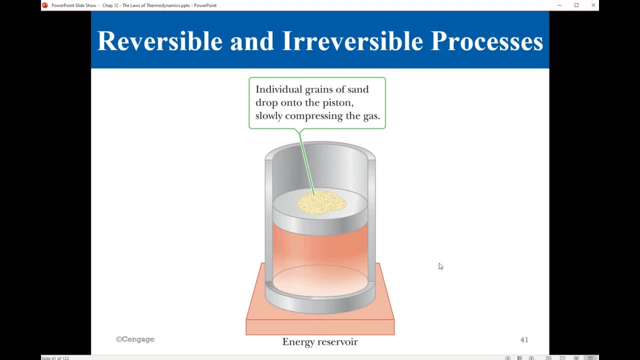 Take a look at this. and the other part is expelled to the environment from the exhaust. can you think of a way to collect the energy release to the environment from the exhaust and bring it back to the system? of course this is impossible, so this process is irreversible. 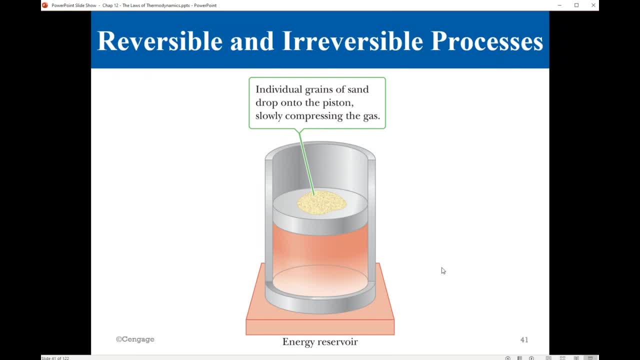 we cannot bring energy release to the environment again to the system cannot go back to the original state. this is irreversible. another example: smoke that is going in the air from a chimney, for example. can we return this smoke back to the previous state? the answer, of course again, is no. most of the processes that occur around 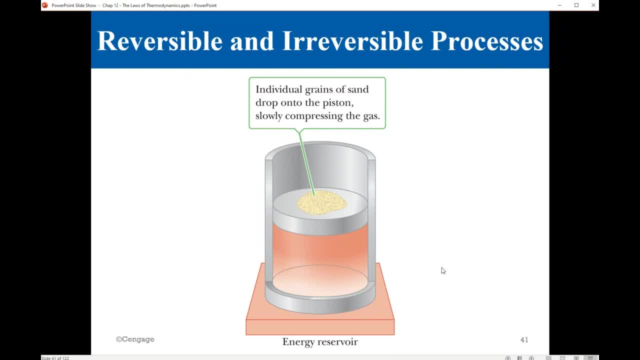 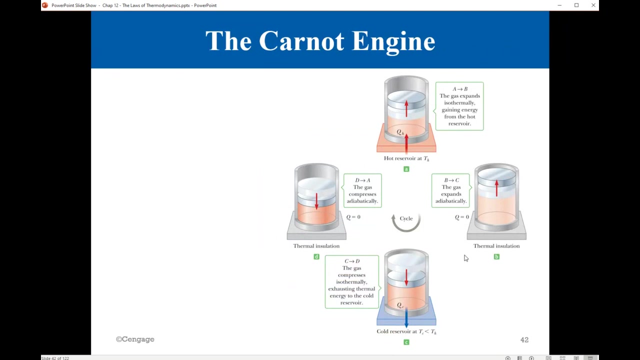 us are irreversible. irreversible processes. you cannot reverse them. a reversible process is an ideal process. okay, it is an ideal process. in real life, most processes that occur in thermodynamics are irreversible. you cannot reverse them. an engineer in france named carnot proposed a model in the 19th century. 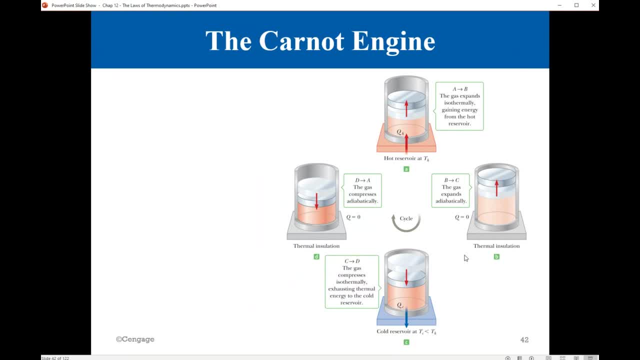 for an engine which now it's called after his name, car root engine. this is an ideal engine. this sets the limit, the upper limit for the efficiency of any heat engine and it allows for reversible processes. as i said, this is theoretical engine, theoretical model. so here we have four phases. we have this state, the gas expands from a to b. 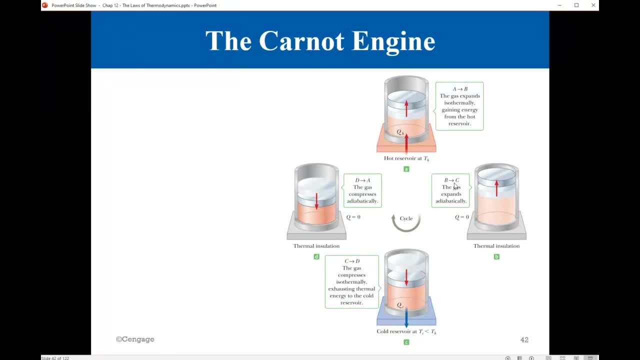 this state. the gas expands diabetically from b to c. the first one was isothermally. the third process, the gas compresses isothermally from state c to state d, and the fourth process: the gas goes back from d to a. so this is the reversible process. 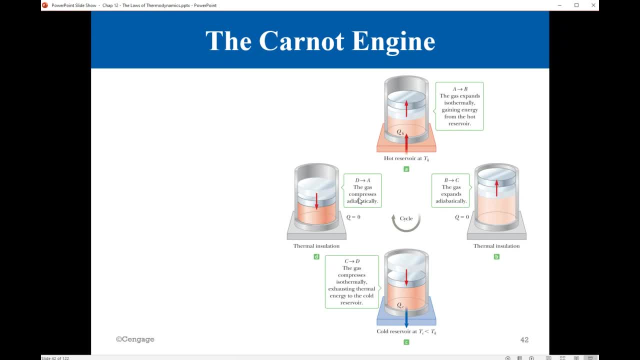 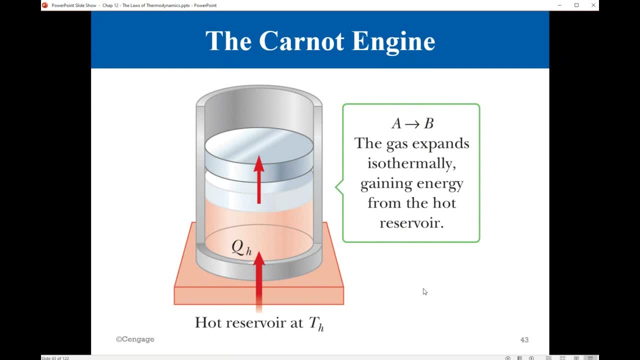 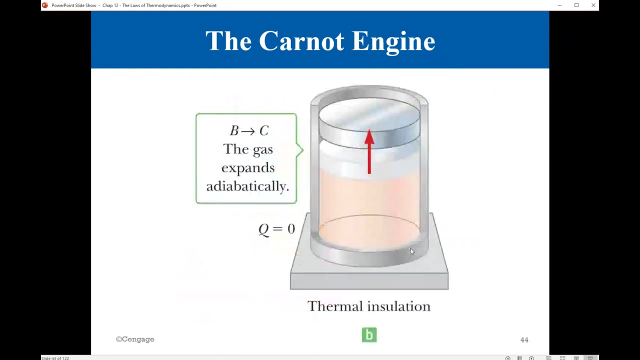 it does that adiabatically here. these four states are outlined in more details here so that we understand this current engine. so this is the first process. the gas expands isothermally, gaining energy from the hot reserve wire and goes from state a to state b. then in the second segment of the cycle, the gas expands adiabatically. 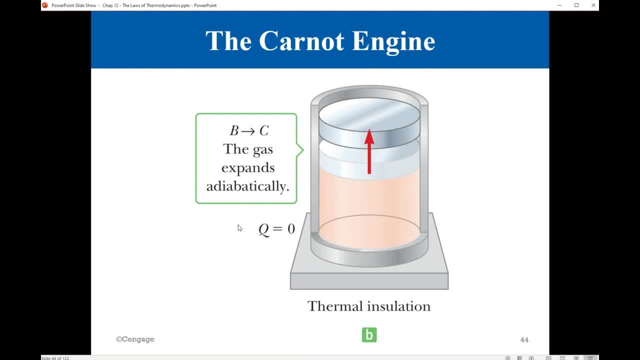 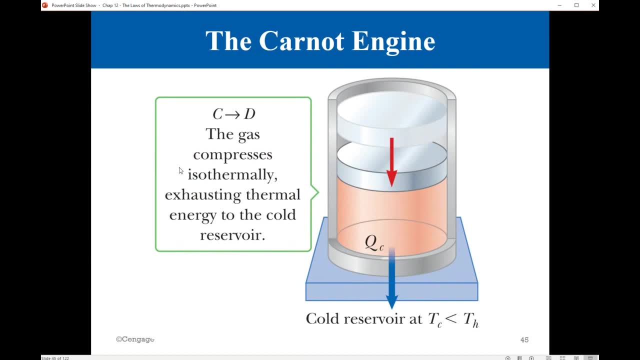 and goes from b to c adiabatically means q is zero. then in the third segment it goes from c to d- the gas compresses isothermally exhausting thermal energy to the cold reservoir. the temperature for the cold reservoir is less than the temperature for the hot reservoir. and in the fourth segment, 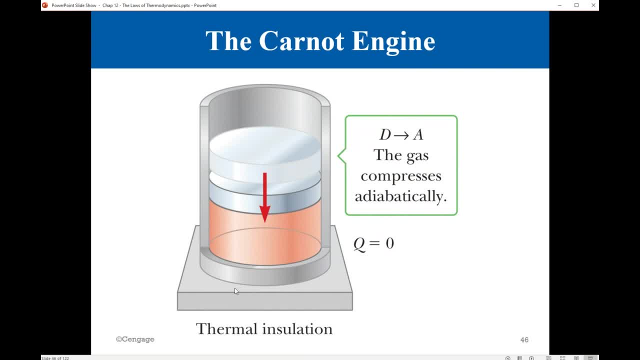 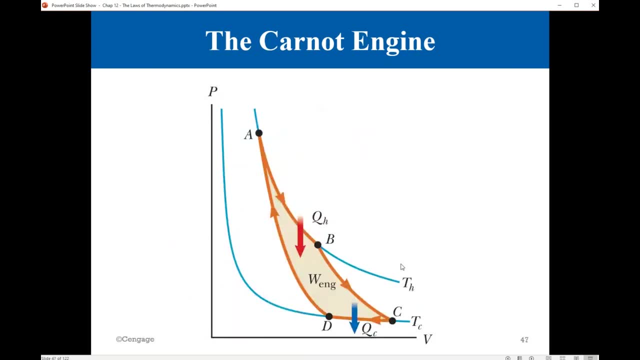 the gas compresses adiabatically goes again from d to a and directly meansq is zero. ADDIEBATICALLY, these are the four processes: from a to b, from b to c, from c to d and fundamentally the gas from C to D, from D to A, So B to C. this is gas expansion adiabatically from D to 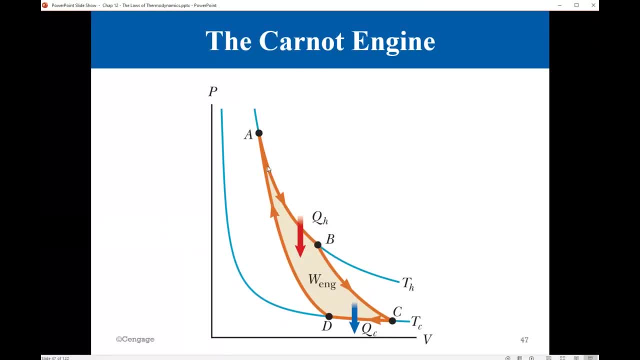 A, this is gas compression, adiabatically from A to B, this is isothermal process, and from C to D, this is isothermal process. So here the system takes quantity of heat from the hot reservoir and here it releases quantity of heat to the cold reservoir. The ratio between 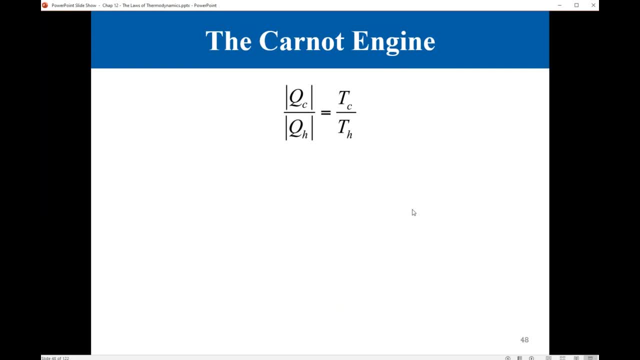 QC and QH is the same as the ratio between TC and TH. So the efficiency that we wrote earlier as one minus QC over QH for the current engine, because QC over QH, this is a corresponding value for one minus QC over QH. so each X2 cube represents Y2 cube. So on X3, there, remains no function of the Zos beggars. So we reduce the function of the Zos beggars. Now, if zos begars are Barbare, If Zos begars fall under Zosthought Uv, This means that somebody 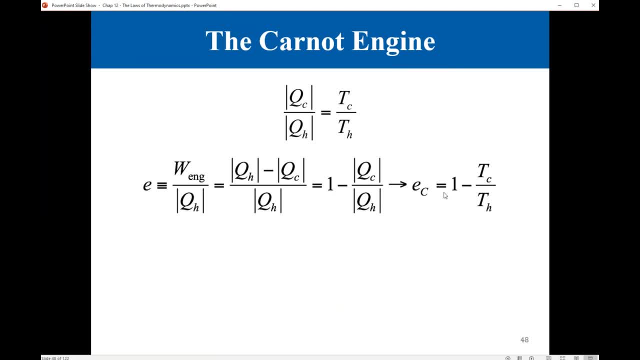 is equal to TC over TH, then we can write the efficiency for a current engine as 1 minus TC over TH. As you can see here, efficiency will always be a fraction. it will never be equal to 1.. So all current engines operating reversibly between the 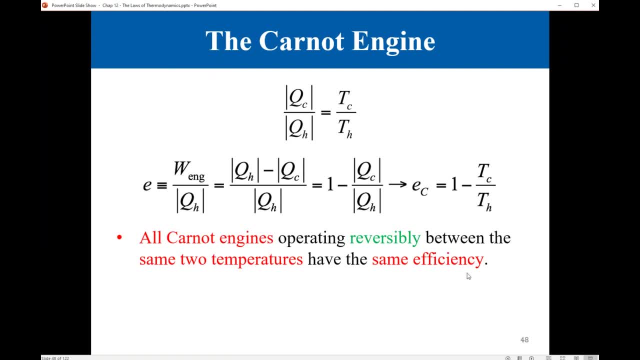 same two temperatures have the same efficiency, because you are dealing with two temperatures. Since the two temperatures are fixed, then the efficiency will be fixed, regardless of what engine you are talking about. Then all real engines operate irreversibly. This is the difference between the. 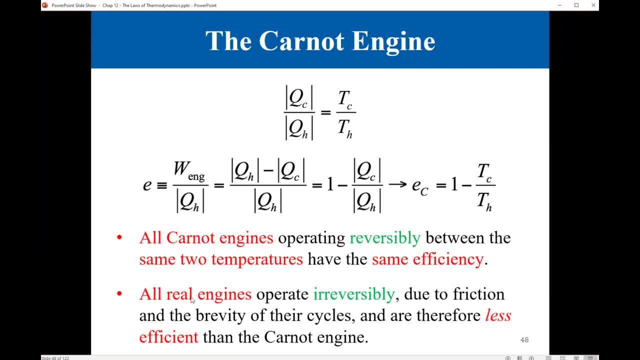 theoretical engine, current engine and the real engines around us. So current engines operate irreversibly, which means you cannot go back to the original state of the system and the efficiency here would be less than the efficiency for a current engine. So a current engine sets an upper limit for the